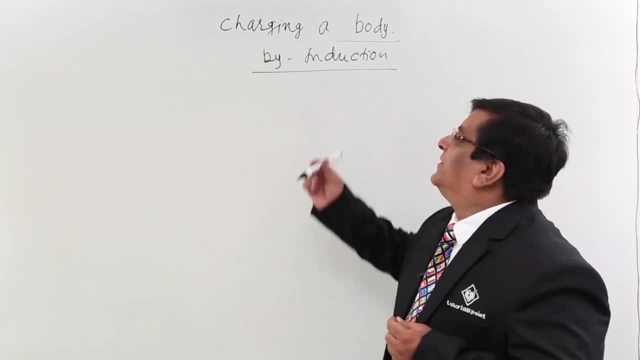 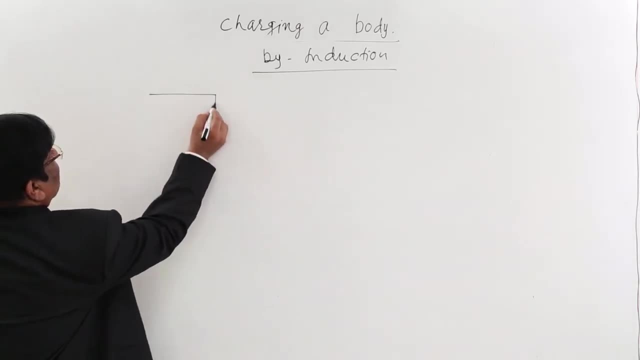 Now we will study how we can charge a body by using the process of induction. Suppose we have a conductor and this conductor is having no net charge. When we say no net charge, I need not to repeat that it is having lot many charges, but the net charge is zero, Equal. 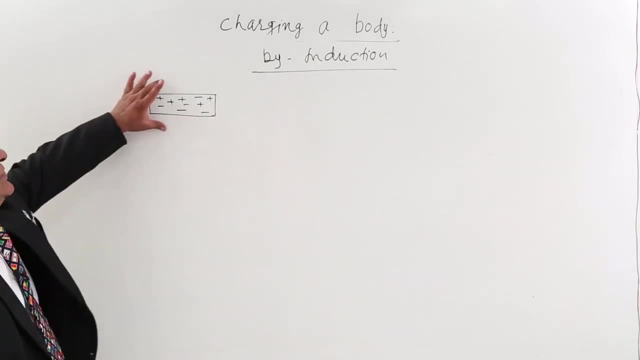 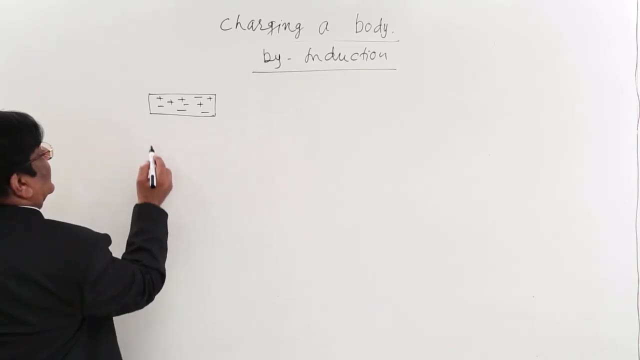 number of positive and negative charges will make it zero charge. Now I want that it should develop certain net charge For that. what do I do? I bring a charged body near it at certain distance. This is a say negatively charged body. If it is a negatively charged, 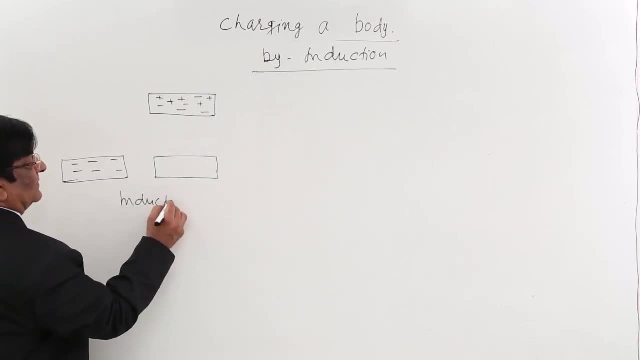 body, induction will take place and in the induction, what we see? that positive charges come here and negative charges are repelled on this side, And plus minus both are here, like this. So this is: induction has taken place. Now, as a third step, this: I connect it with the earth. 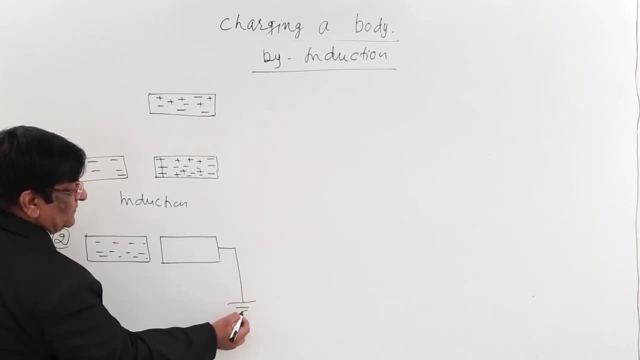 This is symbol of earth. What happens when we connect a body to the earth? The answer is: this is a conductor, and earth is such a big, large body that this can also be taken as a conductor. Now, if this side are axis of electrons, These are being repelled. They 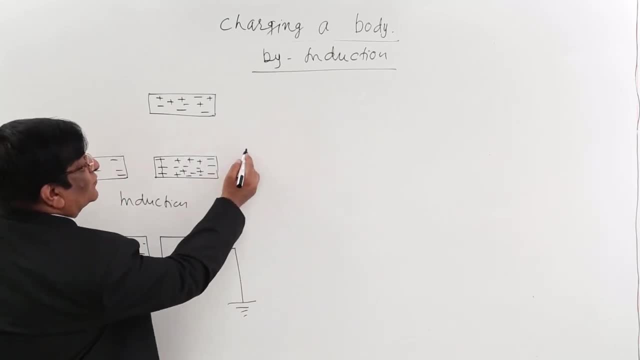 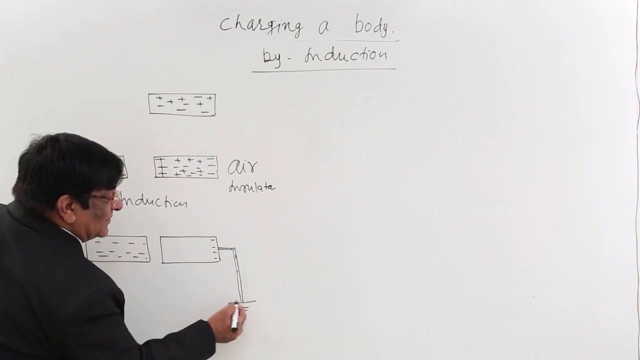 want to move away. They were not able to move away because here is air which is insulator, But now I have connected it with a conductor. They have a passage to move Conductor and this goes to earth and earth is a very large body which is also conductor. So what happens When they?